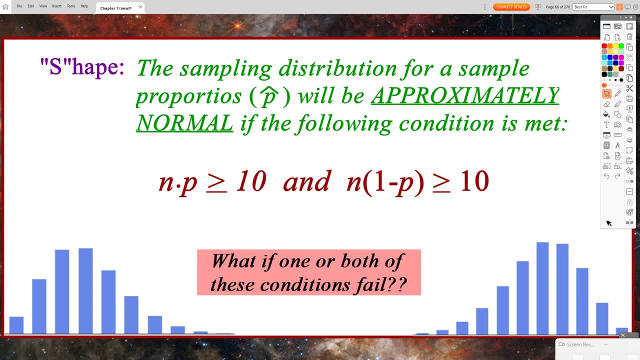 equal to 10.. Now n is our sample size and p is the population proportion, And that was one of the numbers that had to be given to us in the problem itself. So the main question that comes up is what happens if one or both of these conditions? 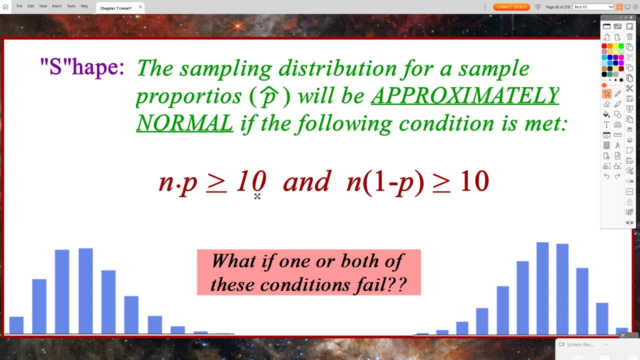 fail. What if I multiply these two values and I don't get a number that's bigger than 10?? Or what if I multiply these values together and I don't get a number that's at least 10?? Well then, that means our sampling distribution for the sample proportions is not approximately. 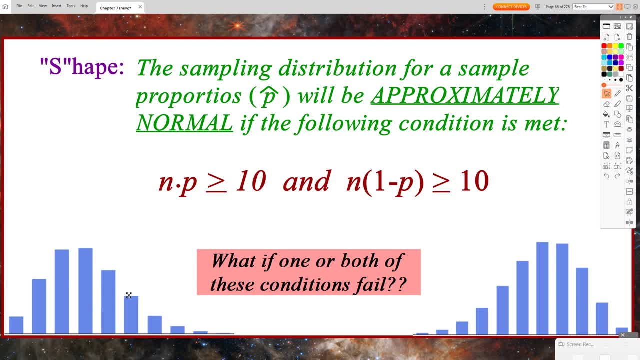 normal And therefore it would have to be either skewed left or skewed right. The main thing you need to know is if this condition fails- and it doesn't have to be both of these fails, but if one or both of them fail, it just means that our sampling distribution. 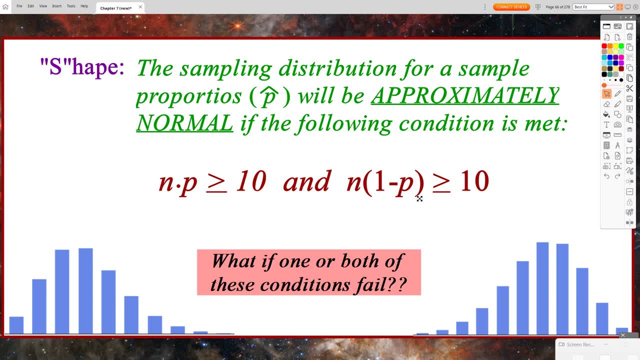 is not approximately normal. That's the main thing. you need to remember that it's just not normal. So what does it look like? if it's not normal? It's skewed in one of the two directions. It just depends on what the value of p is for the most part to know. 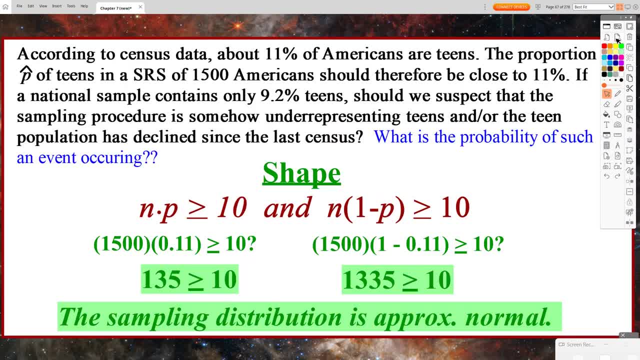 if it's skewed left or skewed right. So for our problem is it approximately normal. So our sample size was 1500.. p the population proportion was the 11%, According to the census data. the census data is taken from the population. 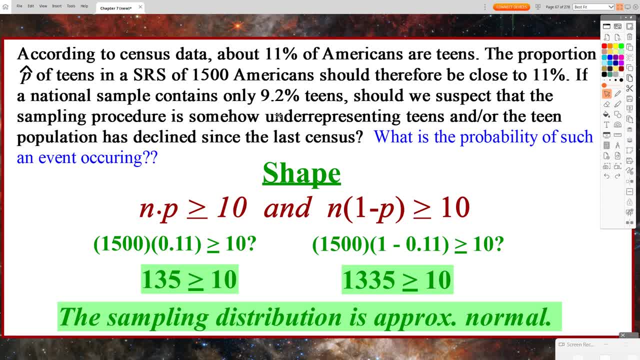 so the 11% is p. Now some people will take the 9.2% as p, but the 9.2% came from a sample and so that would mean that 9.2% is p-hat, not p. 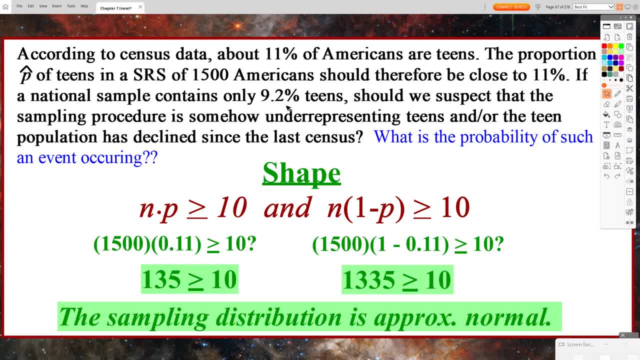 So notice here there is a difference. We do have two proportion numbers. one is a parameter value and one is a statistic value. We need to make sure that we use the right proportion. So 11% for our population proportion, and then we're also going to take 1500 times 1 minus our population. 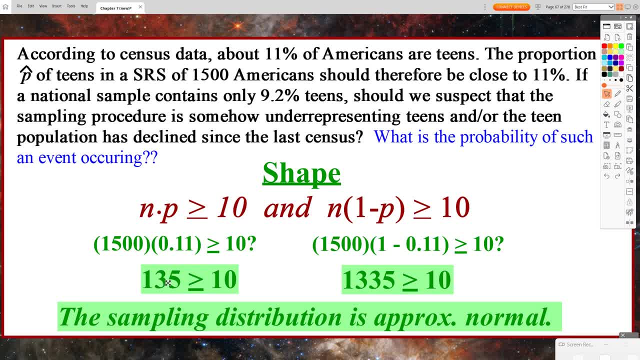 proportion, and when I do the math, I get 135 and 1335, which are both greater than or equal to 10. So I may conclude that the value is an effective number, since we can now use the number to that. the sampling distribution is in fact approximately normal, And that's going to be. 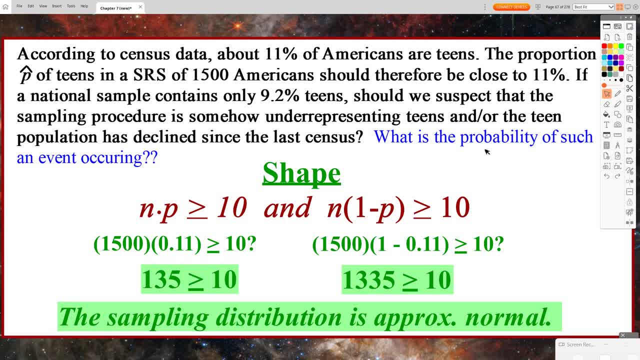 a good thing, because if we want to answer this question, what is the probability of such an event occurring? it would be really nice if our sampling distribution was approximately normal so that we could use- oh, I don't know- normal CDF to calculate the probability of such an event. 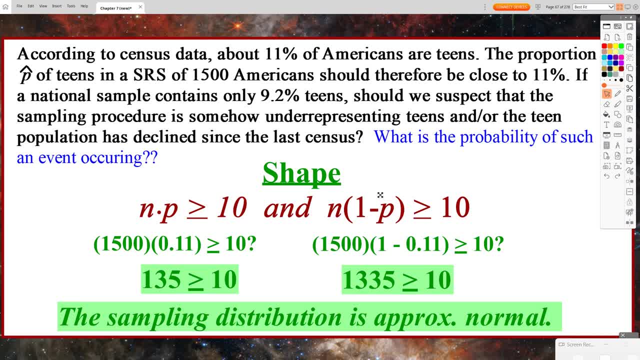 occurring. Now, when you check these conditions, you absolutely need to write pretty much everything out here. Everything that I have highlighted in green is really the main stuff that you absolutely have to have written out Now. one other thing I want to point out is what this n times p and this: 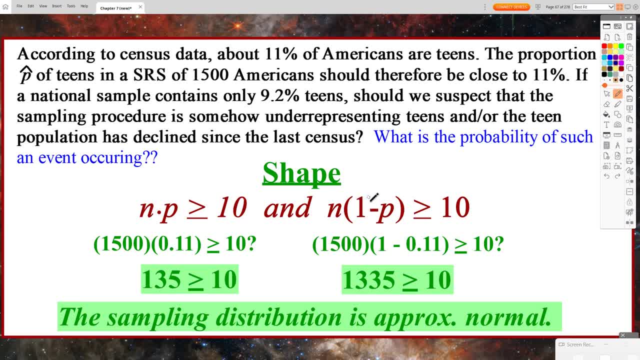 n times 1 minus p really represent. If you think about when we took 1500 times 11 percent, what we're really saying is: out of 1500 Americans and again we're not saying these are 1500 teens. 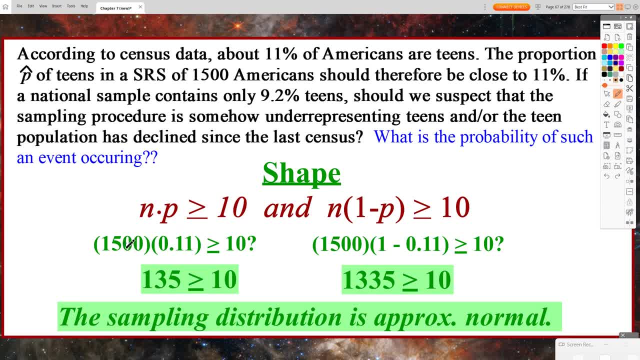 we're just saying we sampled 1500 Americans and we would expect 11 percent of them, according to the census data, to be teens. So this 135 number represents how many teens out of 1500 we would expect to be teenagers. So if you looked at, 135 out of 1500,. that would be the number of teens out of 1500.. So if you looked at 135 out of 1500, that would be the number of teens out of 1500.. So if you looked at 135 out of 1500,. 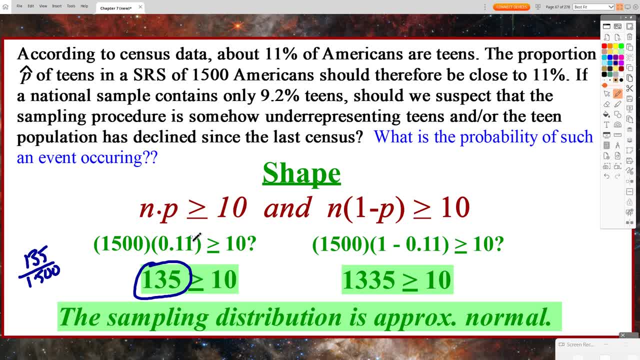 that should give us about 11 percent. Now the other number, the 1335, represents kind of the failures, if you will, people who are not teens. So these could be children that are younger than teenagers, or this could be adults that are older than teenagers. So 1335 represents kind of all the. 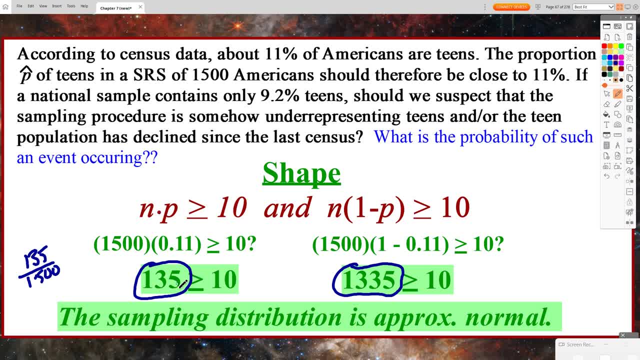 failures. The n times p, the 135, represents our successes. So in a way this is kind of like a binomial distribution or a binomial setting. here We have successes and failures. Now, the other thing I'll just mention here is that these two numbers- since we are discussing a binomial kind, 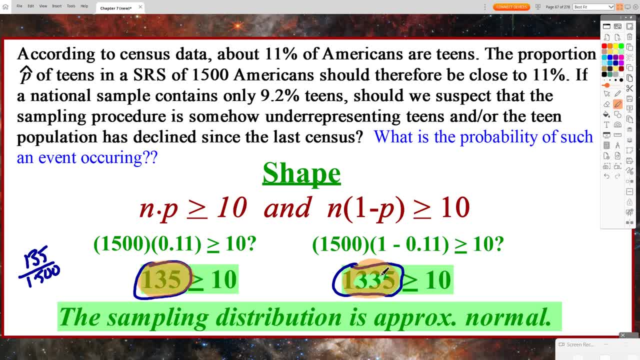 of setting is that these two numbers have to add up to be the total sample size 1500.. So, for instance, if you do this math here and you get 135, you could just say: well, what's the rest of? 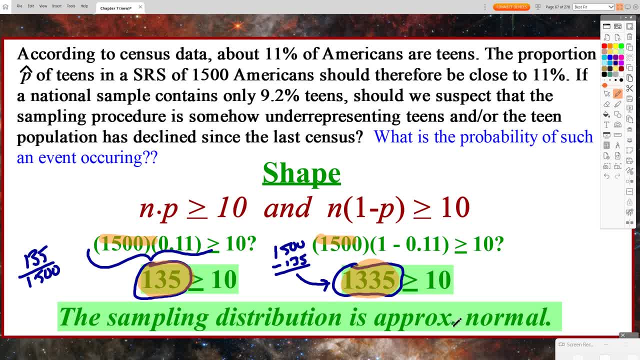 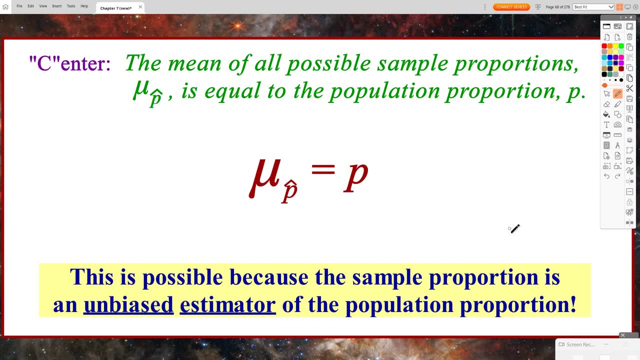 what's 1500 minus this 135, and there's what the other number will end up being. So there's kind of maybe a quicker way that you could get the second number instead of doing the n times 1 minus p formula. Now the center of our sampling distribution for sample proportions, the mean of 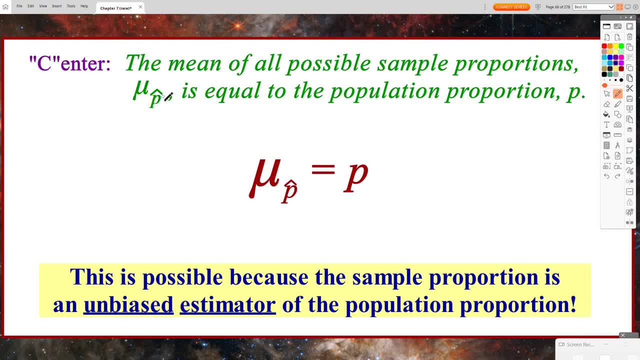 all possible sample proportions: mu sub p hat right. If we took all of these samples and calculated a sample proportion, we would have all of these sample proportions, all of these p hats, creating a sampling distribution, and then what we would find out is that the mean of all of these p hats, the center should be centered right on the true. 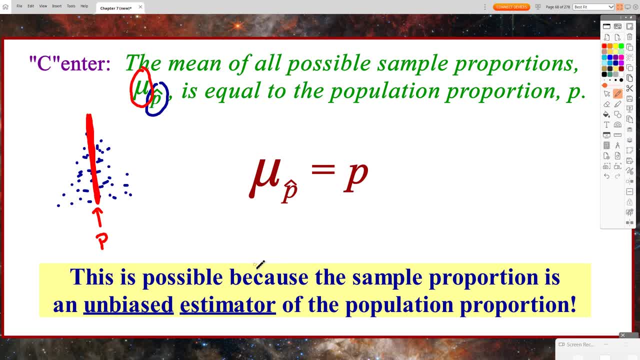 population proportion, which is why the sample proportion is an unbiased estimator of the population proportion. So mu sub p hat, the mean or the center of all possible sample proportions, all of the p hats, of all the sample proportions that we could take, should be approximately the: 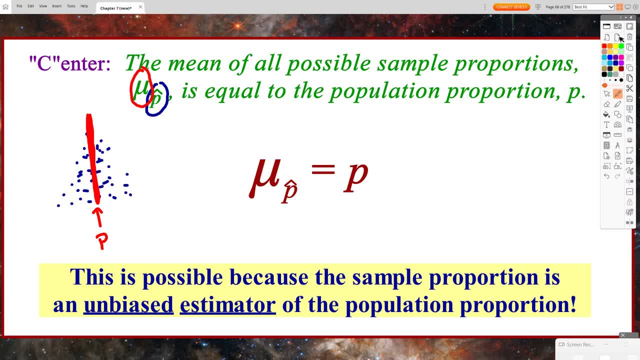 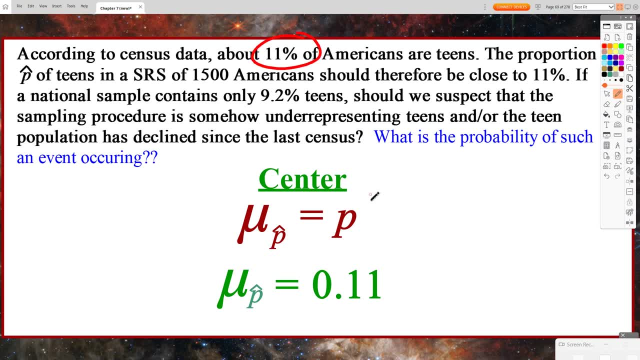 same as the true population proportion. So, for our problem, what would that be? Well, that would be, our 11 percent was what the population proportion value was. Again, this isn't the 9.2 percent. that was the sample proportion. right, That was our sample statistic. that was p hat. 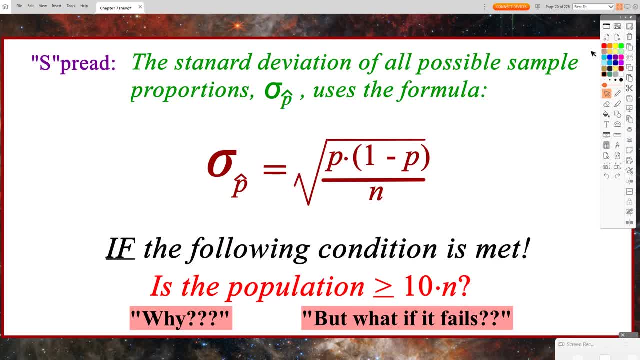 Now, last thing I want to talk about is the sample proportion. So if we take all of the p hats, but not least the spread, the standard deviation of all possible sample proportions, sigma sub p hat uses the formula: the square root of p times 1 minus p, all over the sample size n. Now this one. 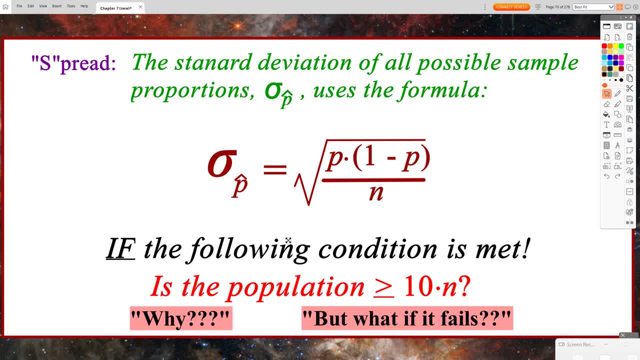 has some baggage tied to it. If the following condition is met- so this is kind of like our shape- we can say the shape is approximately normal if n times p and n times 1 minus p were both greater than or equal to 10.. 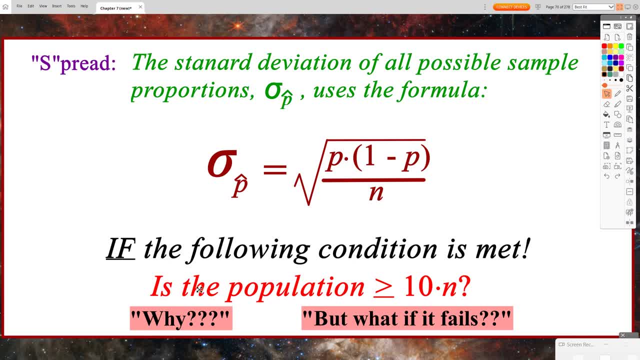 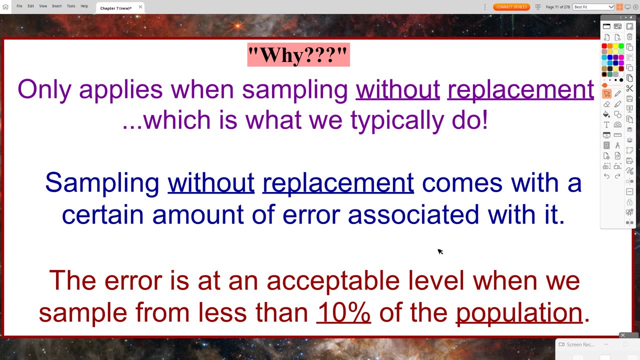 So the condition for the standard deviation is: is the population at least greater than or equal to 10 times the sample size? And you might be wondering: why do we have to have this condition? What if the condition fails? Those are good, valid questions. So first the why, So the condition. 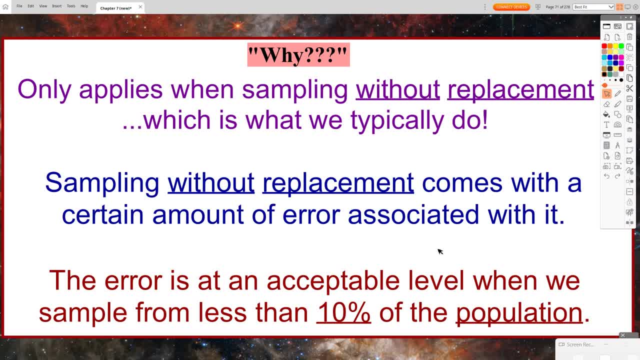 only applies when we're sampling without replacement, which is what we're typically going to do. We're not going to select one person, record their status- if they're a teenager or not a teenager- and then put them back in the population and then sample the next person, because we could get the same person twice. 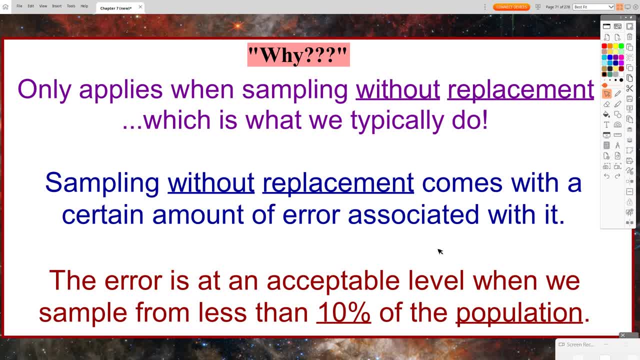 So typically we're not going to sample with replacement. We're typically going to sample without replacement. right, We're going to take one person and then a new person, and then a new person. But as we collect more and more people from our population, our pool of candidates, that 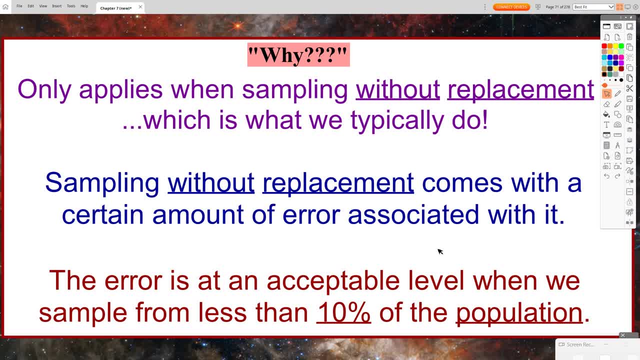 can be next in line, for our sample gets smaller and smaller and smaller. So sampling without replacement comes with a certain amount of error associated with it, And that error is at an acceptable level when we sample from less than 10% of our population. So this condition is also 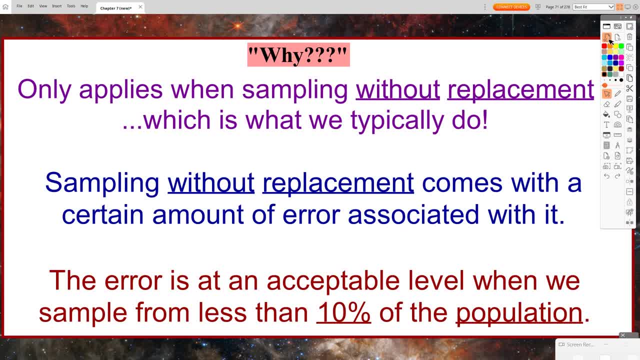 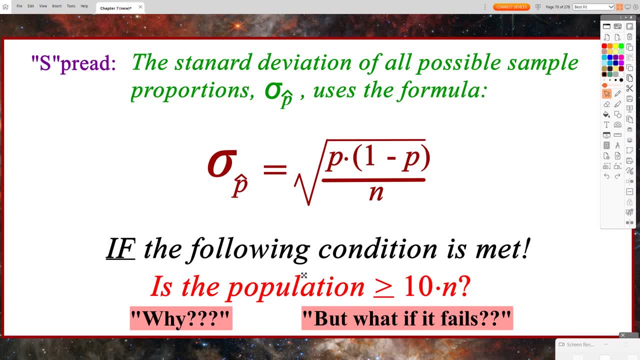 referred to as the 10% rule or the 10% condition come back to here, because our sample size 10 times our sample size. it's got to be smaller than the entire population size. So really this represents less than 10% of our entire population. 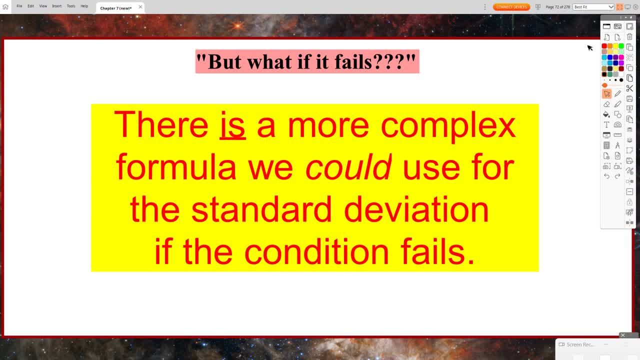 Now what if it fails? What if that condition fails? How are we going to calculate the standard deviation? And the truth is, there is a much more complex formula that we could use for the standard deviation, but we are realistically not going to use that formula in an intro level stats. 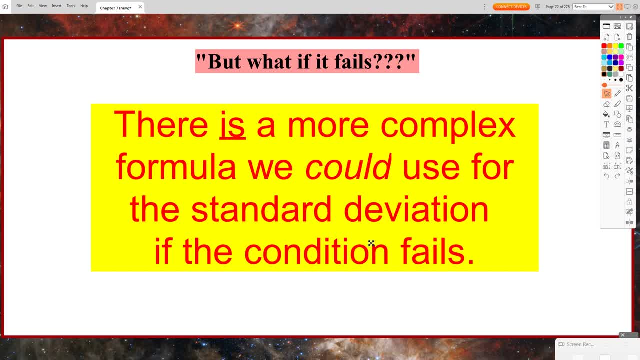 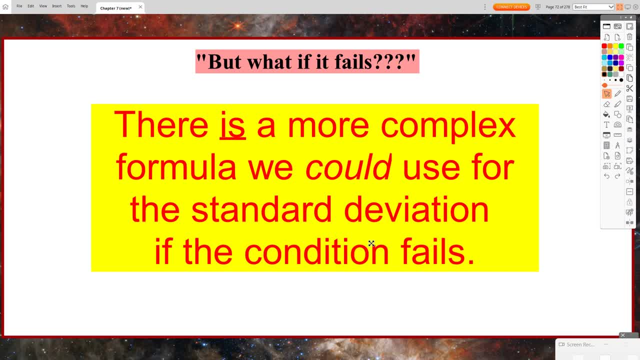 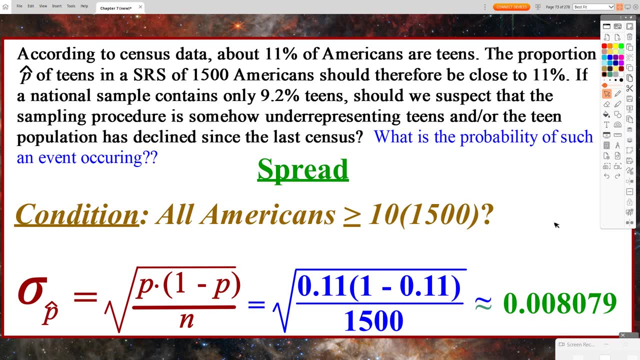 size is, which in some cases you don't really know, So you might have to come up with a good estimate for what that would be. So, for our problem, the population is the population. Who is the population? All Americans, not all teens. We're taking this sample of Americans and determining the proportion. 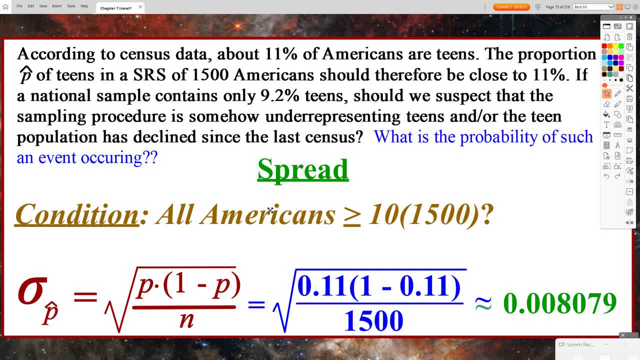 of those Americans that are teenagers. So is our population greater than or equal to 10 times our sample size of 1500?? So 10 times 1500 would be 15,000.. Are there more than 15,000 Americans? 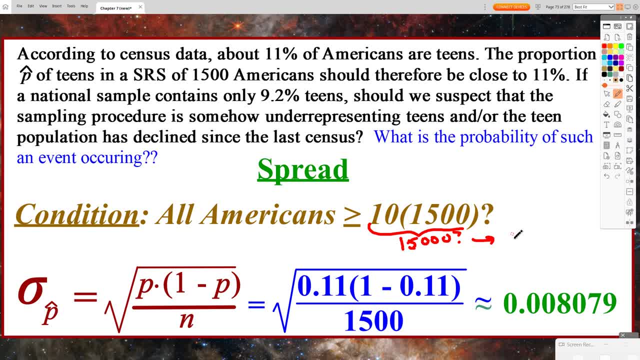 And that would definitely be a scenario where we would say: assume true and not really assume true. I would say: definitely is true, right, Excuse me. So to calculate our standard deviation, I get to use my formula now, And so I plug in 0.11,, 11% in for the population proportion. 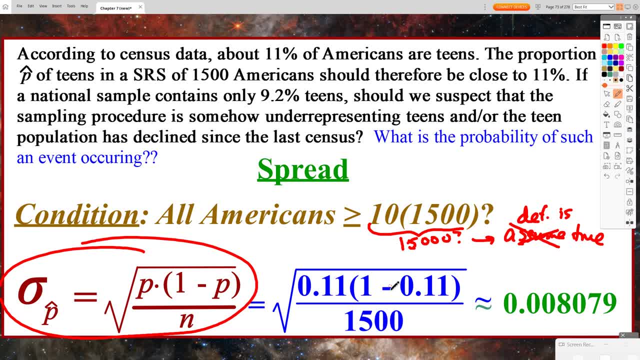 And I divide that p times 1 minus p, divided by the sample size of 1500, square root that value and I get a number that is just under technically 1%. It's 0.8% is our standard deviation. 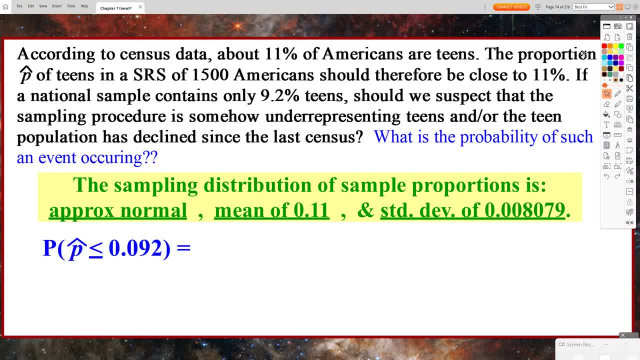 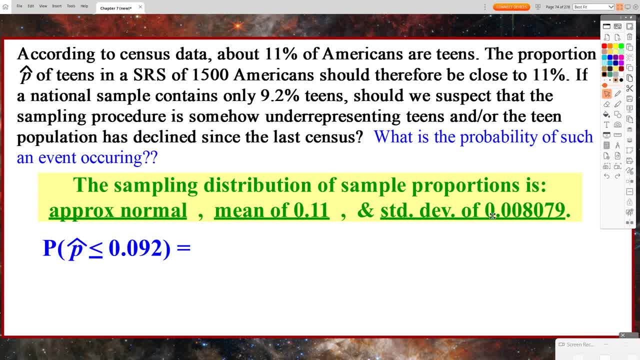 legen slightly smaller than 1% at 0.8079%. So now we can finally get to the question that we really asked here: what is the probability of such an event occurring? Well, what was that event that occurred? we took a sample and we found in our sample: 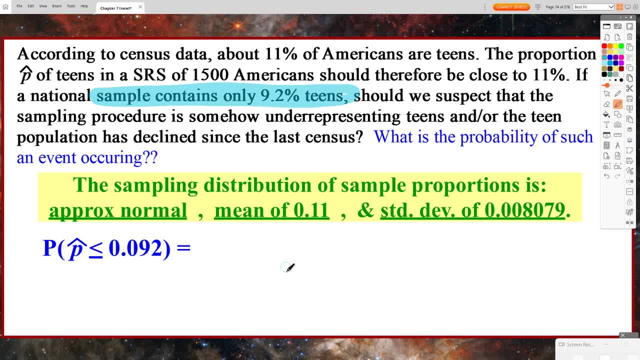 only 9.2% of teens. So what is the probability? Qué? so let's kinda colour code and match things up here. what is the probability? so capital P of such an event. What was our event? We had a sample. 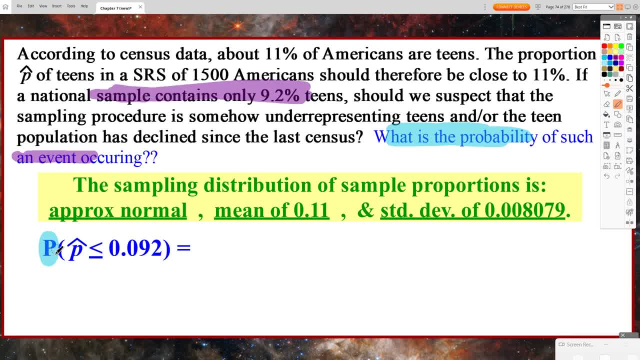 proportion. that was 9.2.. So our sample proportion, our p-hat, was 9.2%. Now you might be wondering why did I put less than or equal to, Why didn't I put equal in this scenario? Because that was. 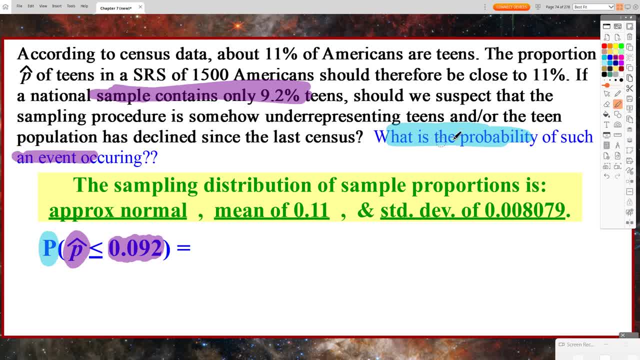 the event that occurred, that p-hat was equal to 9.2%. Well, if you consider, we have an approximately normal distribution, which is a continuous distribution, And so the probability of a single value happening in an approximately normal distribution is roughly 0%. So we need to. 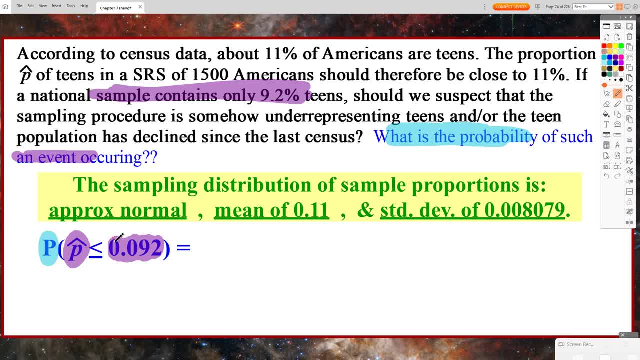 give our approximately normal distribution an area to consider And since our 9.2% was less than what we expected to happen at 11%, then we're going to consider everything that happens on that left end of the distribution. So if I were to draw a picture of what's happening, 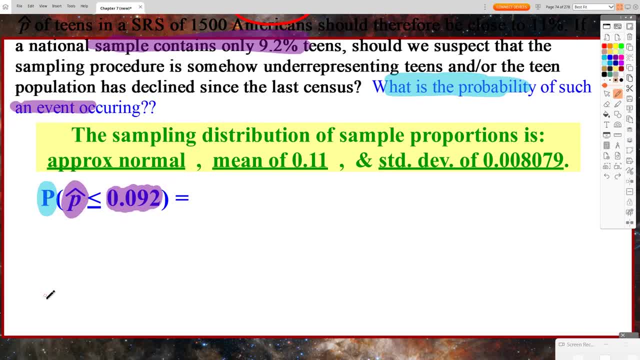 here I've got an approximately normal shape. I know the mean in the middle mu sub p-hat. is that 11%? And we saw something that was less than 11%. We saw. here's our p-hat of 0.092.. And again, if I wanted to just do 0.092, what is its probability? 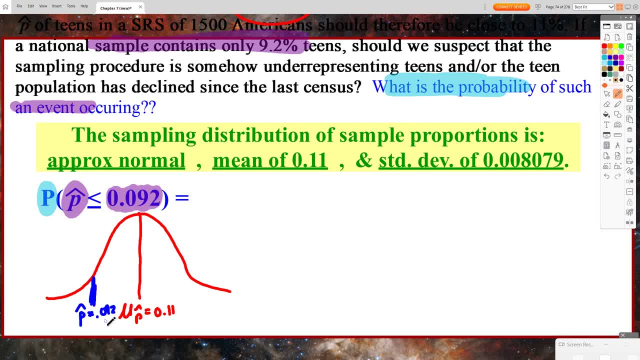 I'm really finding the area of a segment which is roughly 0.. So if I'm already on the left side of the distribution to give that 9.2% really any kind of value, I need to figure out what is the probability of that event occurring or other more probable events that are occurring. So if I'm 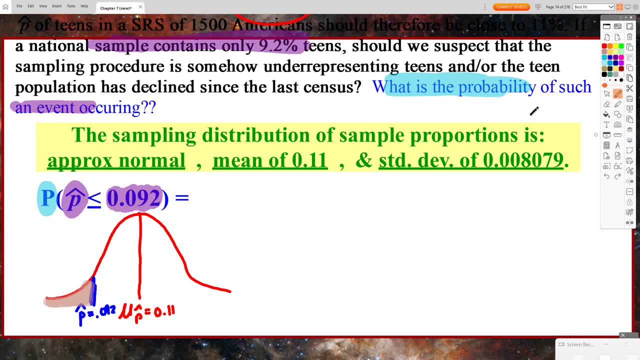 just drawing a picture of a segment. what is its probability of that event occurring or other rare events occurring? So we will get to use normal CDF because we verified that the shape is approximately normal. Our lower bound would be realistically 0, or theoretically we can do negative infinity. 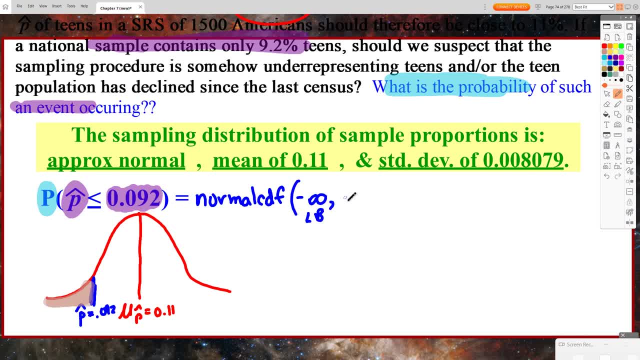 as our lower bound. Our upper bound is the 9.2%, Our mean. what we expected to see happen was our 11% And our standard deviation was the 0.008079.. And so once we throw that into our normal CDF, we're going to get what is the probability of seeing such an event occur? 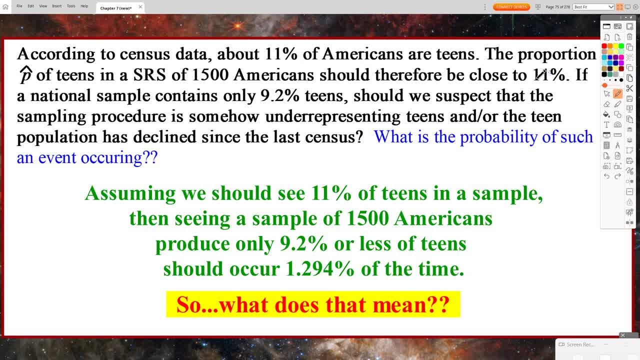 And that answer is 1.294%. So normal CDF is going to give us really 0.01294.. Now what that number initially represents is saying: assuming that we should see 11% of teens in a sample, then seeing a sample of 1,500 Americans produce only 9.2% or less of teens should occur about 1.294% of the time. 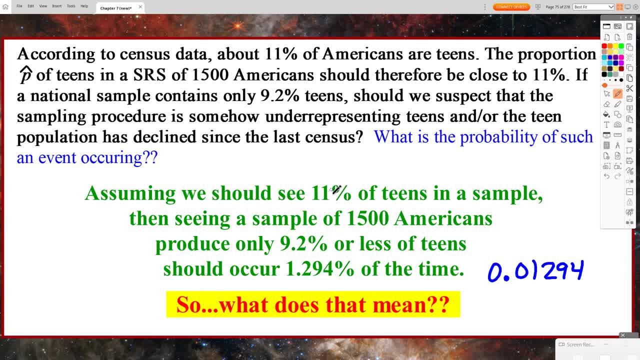 So what exactly does that mean? There were a couple ideas up here in the question that we were exploring. Should we suspect that the sampling procedure is somehow under-representing teens, And or has the teen population declined since the last census? So, taking those two things into account, what we're really kind of pondering and considering here is: 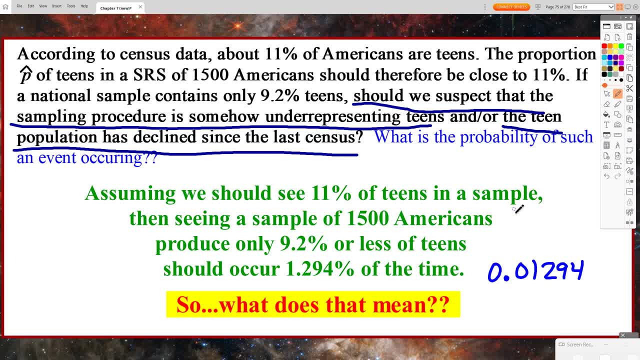 number one. we could have just gotten a sample, A sample of 1,500 Americans- that had not so many teens in it, less than what we would have expected- And that could happen. That's just sampling, variability at its finest. We're not always going to get 11% of teens in every single sample that we get. 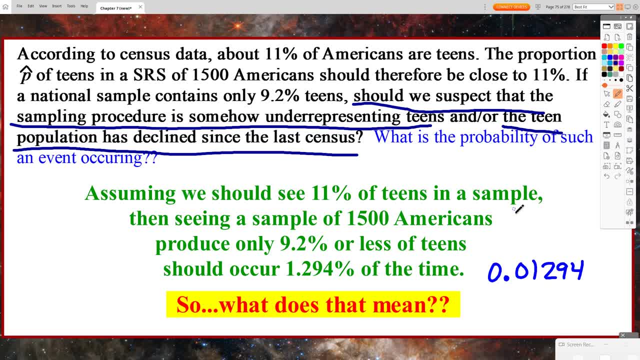 Some of them are going to have more teens. Some of them will have less teens. We just happened to get a sample that maybe had less teens, So that's one thing that could have happened here. The other thing that could have happened is: 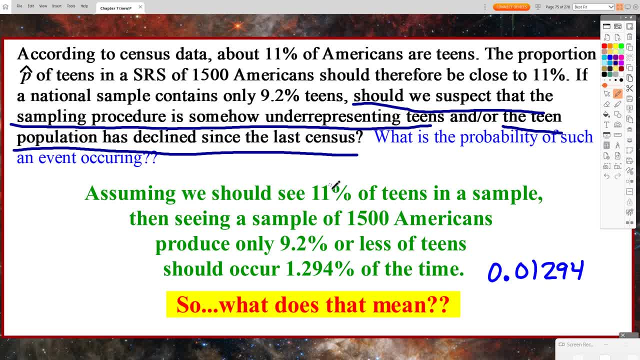 maybe the truth about the population is that it's no longer 11% teens, Maybe it's something closer to 9.2%. Maybe the population has declined for teenagers, We don't know. So which of those two scenarios is the truth? 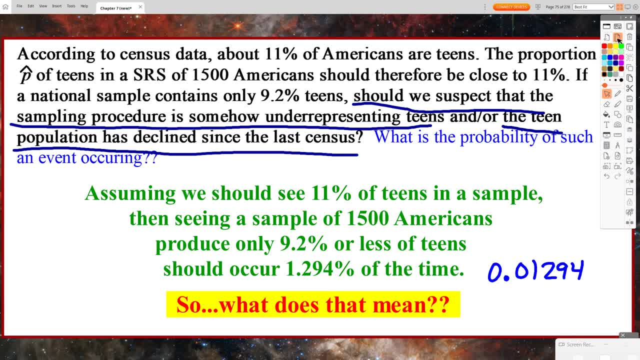 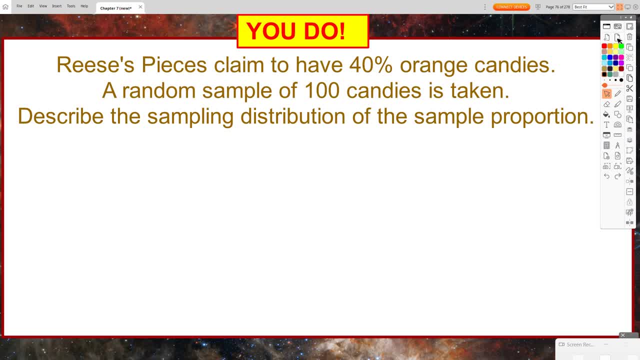 We just don't know. So what I want you to consider is that Reese's Pieces claim to have 40% orange candies. A random sample of 100 candies is taken. I want you to describe the sample, The sampling, distribution of the sample proportion. We will discuss this the next day in class.